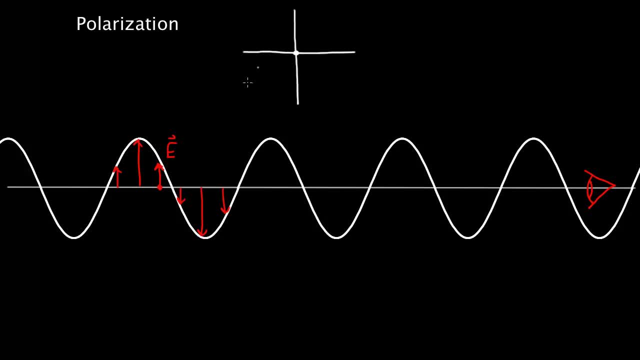 so imagine we're looking straight down that line and then up and down is up and down, and then left and right. that direction I have the magnetic field would be this way and that way. What would my eye see? Well, my eye's only gonna see electric fields. 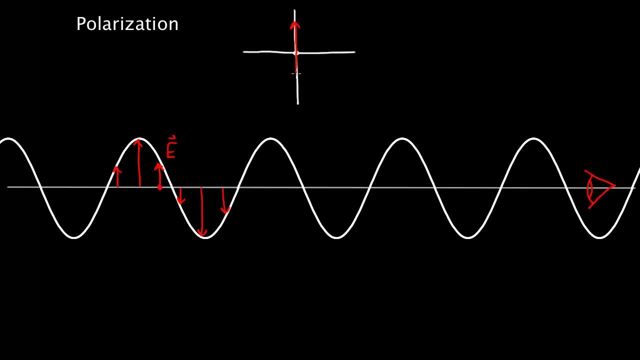 that either point up or electric fields that point down. They might have different values, but I'm only gonna see electric fields that point up or down. because of that, this light ray, this light ray, is polarized, so polarized light is light. 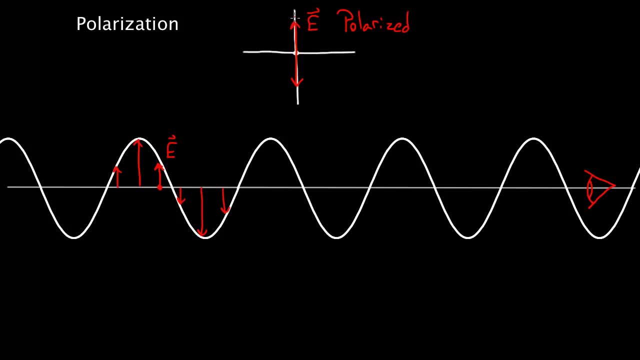 where the electric field is only oscillating in one direction- up or down. that's one direction vertically, or it could be polarized horizontally, or it could be polarized diagonally, but either way you could have this wave polarized along any direction. 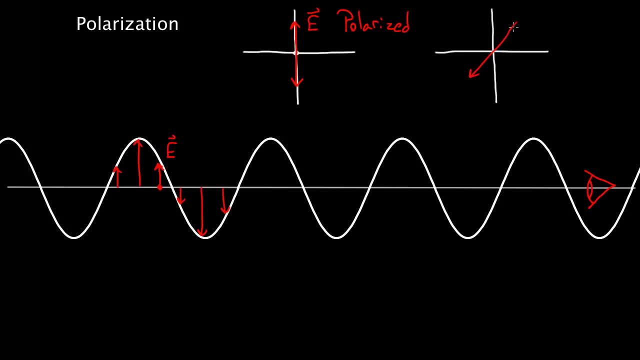 I mean a light ray like this, if we had it coming in diagonal, this light ray that's oscillating like this, where the electric field oscillates like that, that's also polarized. these are both polarized because there's only one direction. 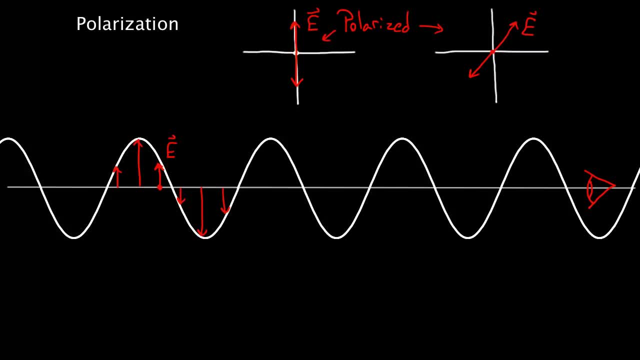 that the electric field is oscillating in and you might think: well, how could you ever have a light ray that's not polarized? Easy, most light that you get is not polarized, that is to say, light that's coming from the sun. 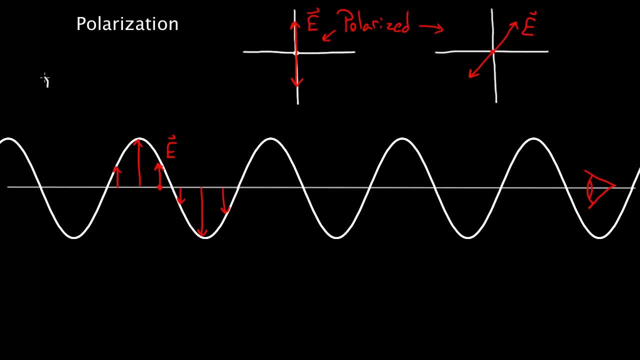 straight from the sun, typically not polarized light from a light bulb, an old incandescent light bulb- this thing's hot. you can get light polarized in any direction Once all overlapping. so if we draw this case for a light bulb, just a random incandescent light bulb. 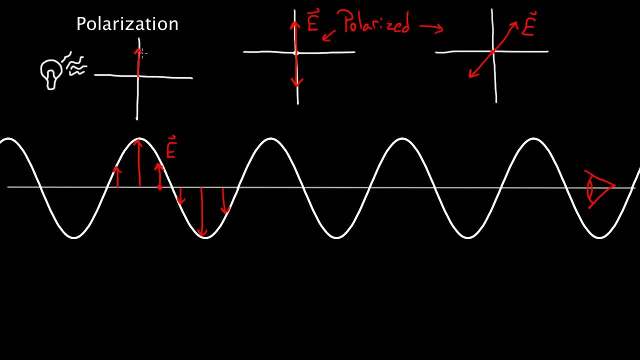 you might get light. some of the light hitting your eye you can get some light. that's got that direction. you got light. that's got this direction. you got light in all these directions at any given moment. I mean you'd have to add these up. 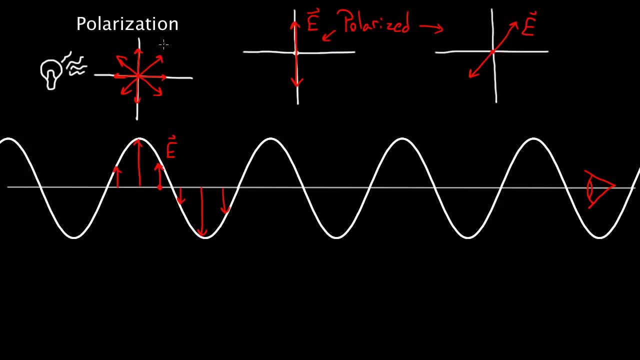 to get the total, and they might not all be the same value. but what I'm trying to say is: at any given moment, you don't know what direction the electric field's gonna be hitting your eye at from a random source. it could be in any direction. 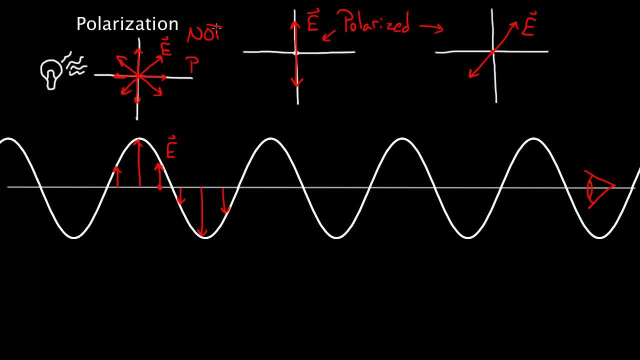 so this is not polarized. This diagram represents light that is not polarized. At some point the field might be pointing this way. at some later point it's this way. it's just random. You never know which way the electric field's. 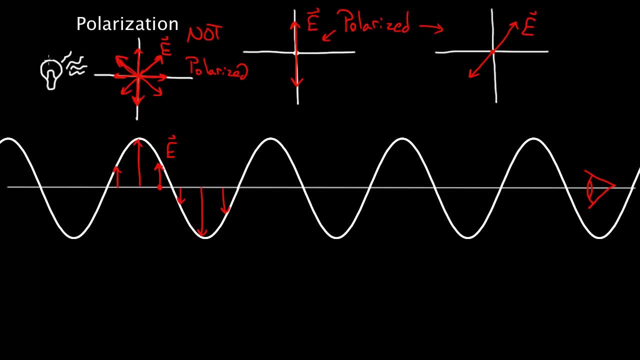 gonna be pointing, whereas these over here, these are polarized. so how could you polarize this light? Let's say you wanted light that was polarized. You were doing an experiment, you needed polarized light. well, that's easy: you can use what's called a polarizer. 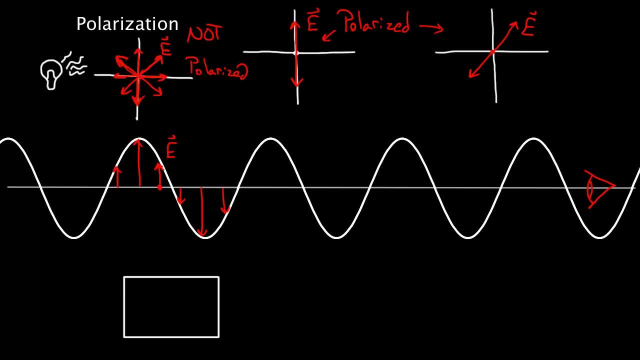 and this is a material that lets light through, but it only lets light through in one orientation. so you can have a polarizer that, for instance, only lets through vertically polarized light. so this is a polarizer. these are cheap. 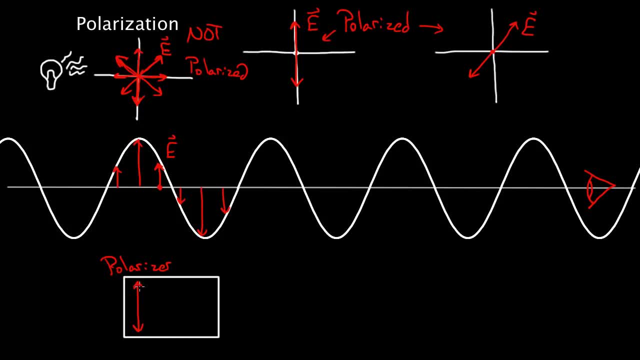 thin plastic configured in a way so that it only lets light through that's vertically polarized. Any light coming in here that's not vertically polarized gets blocked or absorbed. so what this means is, if you use this polarizer and held it in between your eye, 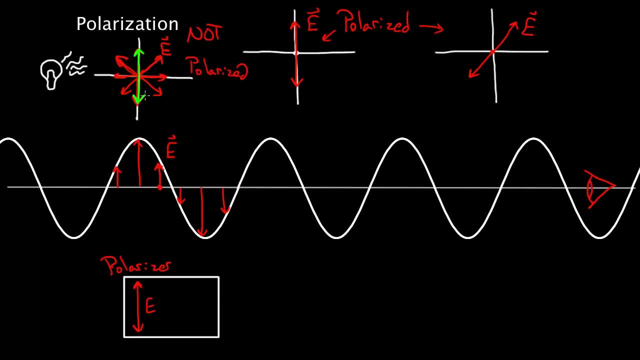 and this light bulb, you would only get this light. All the rest of it would get blocked. Or you can just rotate this thing and imagine a polarizer that only lets through horizontal light. Now, it would only let through light. that was this way. 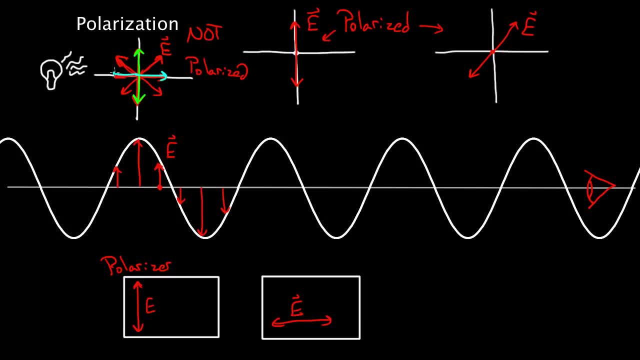 and so you would only get this part of the light, or you could just orient it at any angle you want and block everything but the certain angle that this polarizer is defined as letting light through. So you can do this, and once you hold this up, 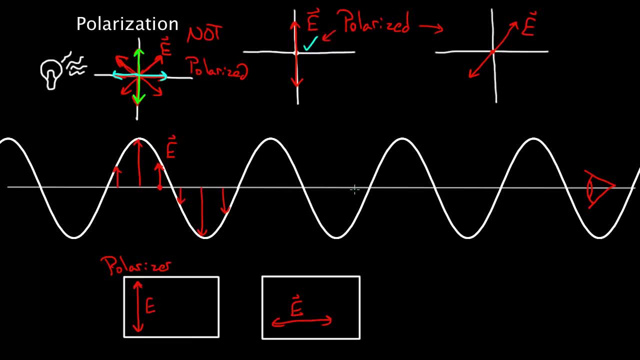 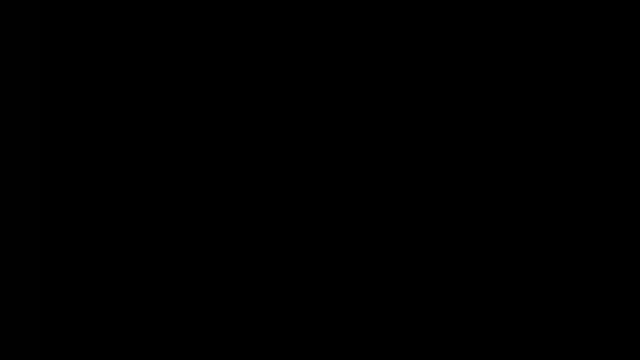 you get polarized light, light that's only got one orientation. so that's what polarization means. But why do we care about polarization? Well, let me get rid of this for a minute. You've heard of polarized sunglasses, so imagine you're standing near water. 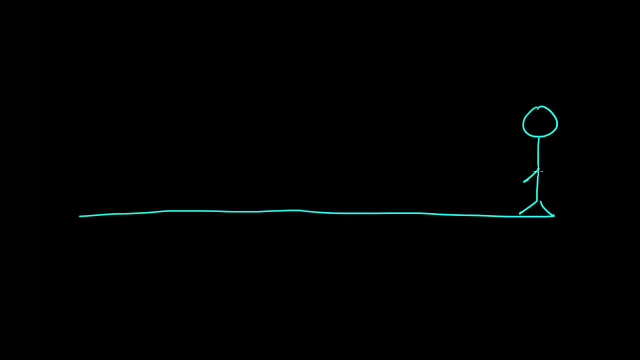 or maybe you're standing on ice or snow or something reflective. there's a problem. Say the sun's in, It's out, it's shining, it's a beautiful day, except there's gonna be glare. Let's say you're looking down at something here on the ground. 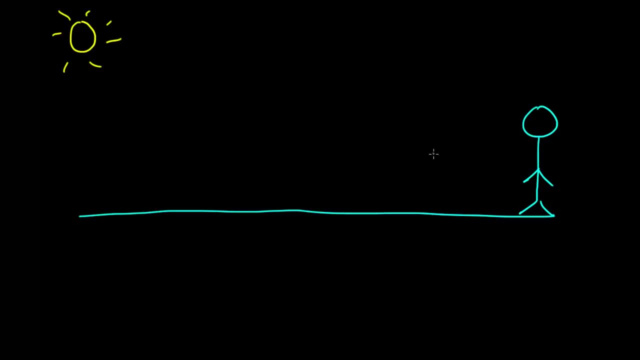 Well, it's gonna get light reflecting off of it from just. you know. light's coming in from all directions, but it also gets this direct light from the sun, So it gets light from reflected off the clouds and whatever's nearby ambient light. 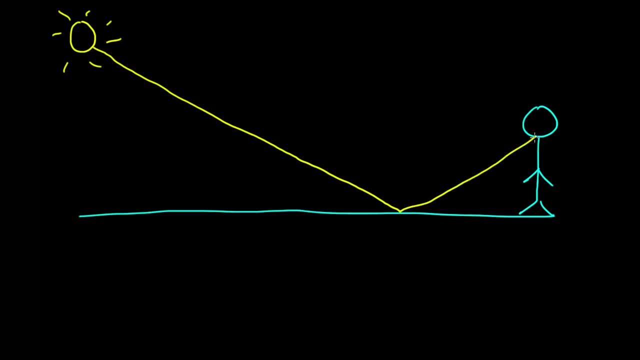 And then there's also this direct sunlight that's harsh. If that reflects straight up to your eye, that hurts. We don't like that. It blocks our vision, it's hard to see, it's glare. We don't want this glare. so what can we do? 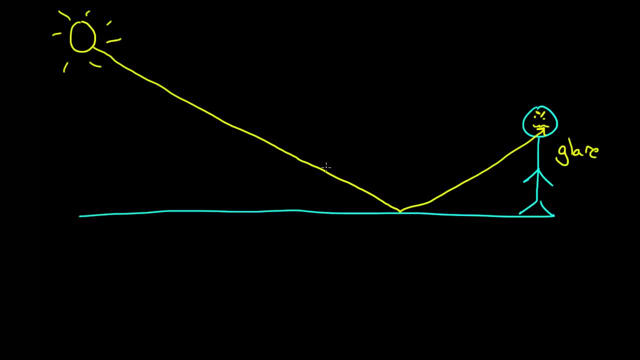 Well, it just so happens that when light reflects off of a surface, even though the light from the sun is not polarized, once it reflects it does get polarized, or at least partially polarized. So this surface here, once this light reflects, 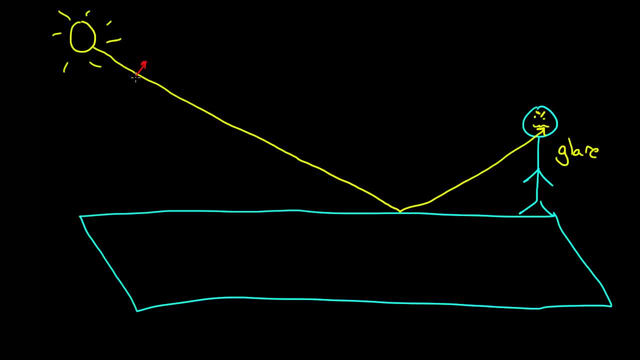 it's coming in at all orientations. You got electric field. you never know what electric field you're gonna get straight from the sun. And when it reflects, though, you mostly get upon reflection the direction of polarization defined by the plane of the surface that it hit. 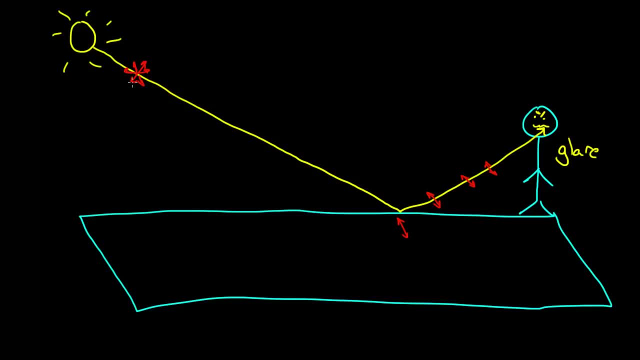 So, because the floor is, you know, horizontal, when this light ray hits the ground and reflects that reflected light, gets partially polarized, This horizontal component of the electric field is gonna be more present than the other components. Maybe not completely, sometimes it could be. 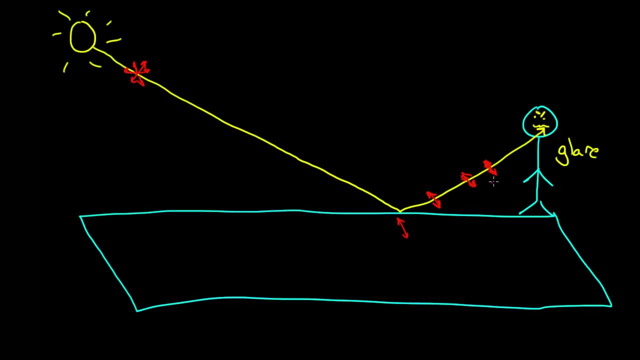 It could be completely polarized, but often it's just partially polarized. But that's pretty cool, because now you know what we can do. I know how to block this. We just get some sunglasses, We put some sunglasses on and we make our glasses. 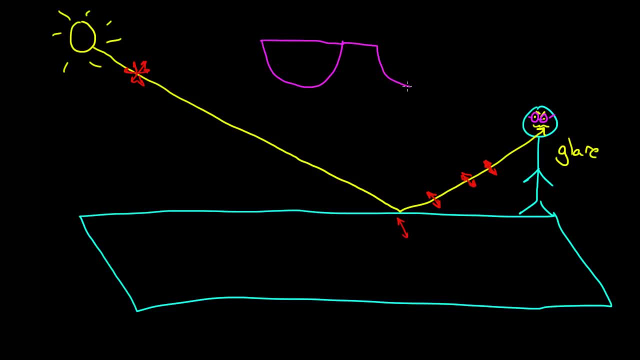 so that these are polarized. and which? how do we want these polarized? I want to get rid of the glare, So what I do is I make sure my sunglasses only let through vertically polarized light. Here's some polarizers. 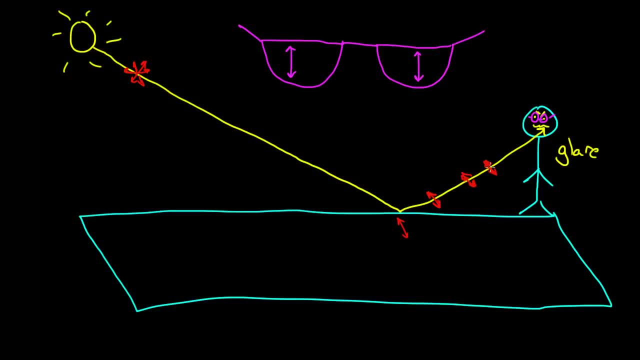 That way a lot of this glare gets blocked because it does not have a vertical orientation, It has a horizontal orientation and then we can block it. So that's one good thing that polarization does for us. in understanding it, we can get rid of glare. Also fishermen like it because if you're trying to look in the water at fish, you want to see in through the water. You want to see this light from the fish getting to you. You don't want to see the glare off of the sun getting to you. 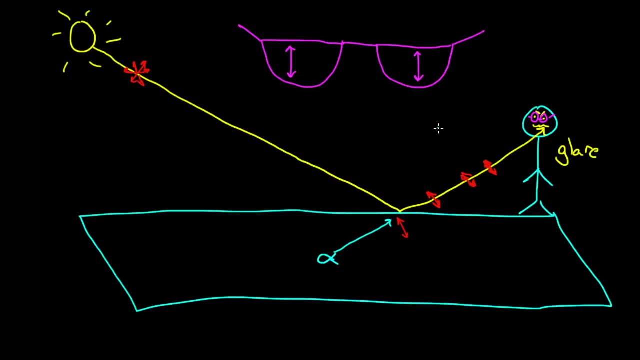 So polarized sunglasses are useful. Also, we can play a trick on our eye. if we really wanted to, You could take one of these. make one eye, have a vertical orientation for the polarization, have the other eye with a horizontal, and you're thinking this is stupid. 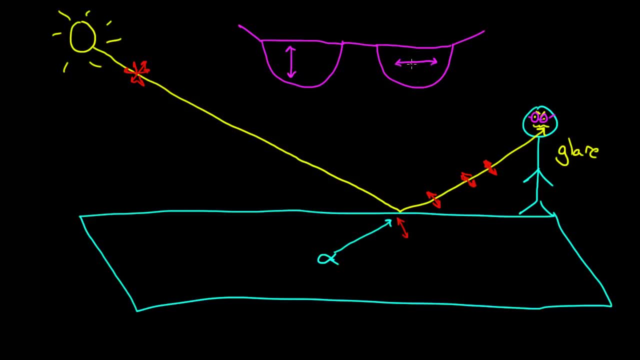 What would you do this for? This eye's going to get a lot of glare. Well, you wouldn't use that. You wouldn't use these outside when you're like skiing or fishing, but you could play a trick on your eyes If you went to the movies and you went and watched a movie. 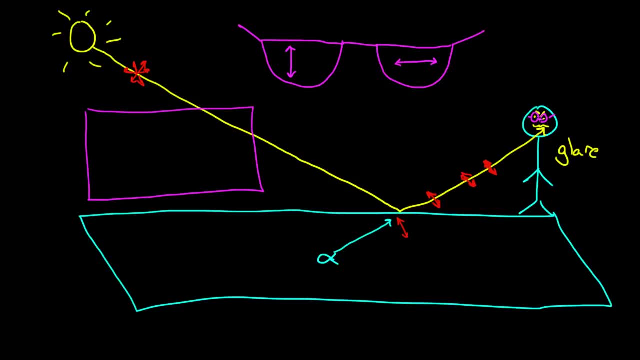 well, the reason our eyes see 3D is because they're spaced a little bit apart. They each get a different, slightly different image That makes us see in 3D. Well, we can play the same trick on our eye if we have the polarization, like this: 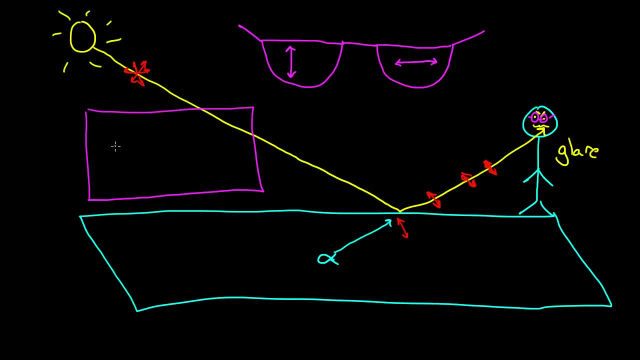 If light, if some of the light from the movie theater screens coming in with one polarization and the other light's coming in with the other polarization, we can send two different images to our eyes at the same time. If you took these off, it'd look like garbage. 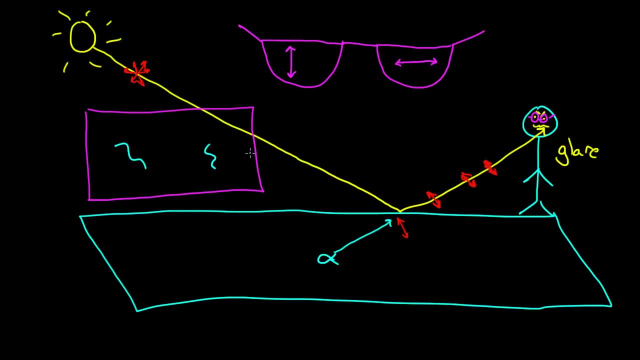 because you'd be getting both of these slightly different images. It'd look all blurry, and it does. If you take off your 3D glasses and look at a 3D movie, it looks terrible because now both eyes are getting both images. but if you put your glasses back on, 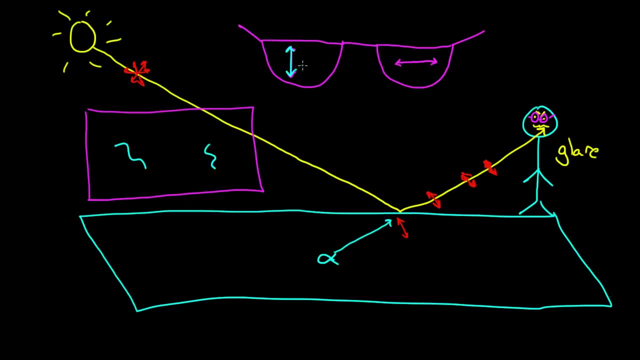 now this eye only gets the orientation that it's supposed to get, and this eye only gets the orientation that it's supposed to get, And you get a 3D image. So it's useful in many ways. And let me show you one more thing here. 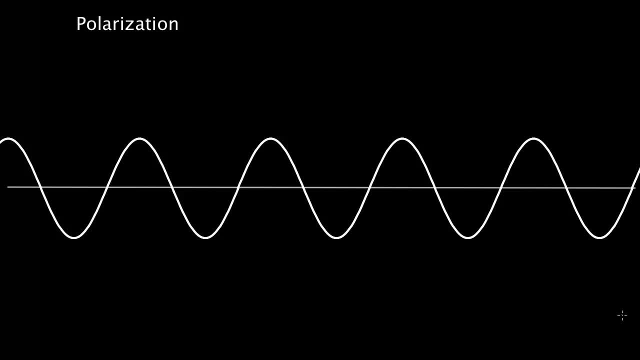 Let's come back to here. This light was polarized vertically and so that's called linear polarization. Anytime same with these. These are all linear polarization, because just up and down one linear direction, Just diagonal. this is also linear. 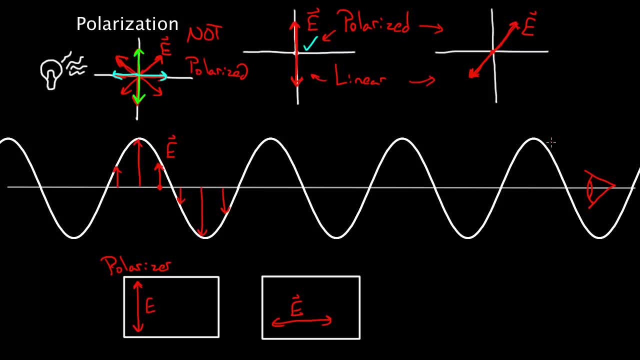 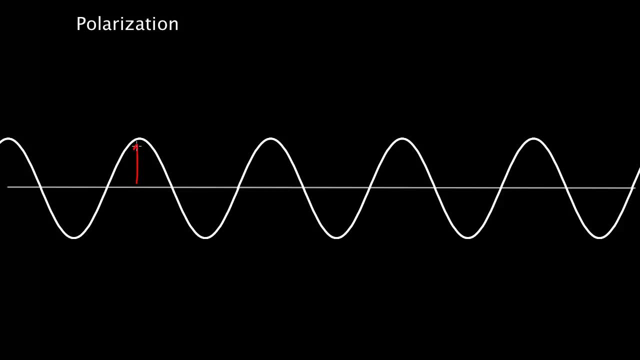 All of these are linear. You can get circular polarized light. So if we come back to here, we've got our electric field pointing up like that. Now let's say, we sent in another light ray, another light ray that also had a polarization. 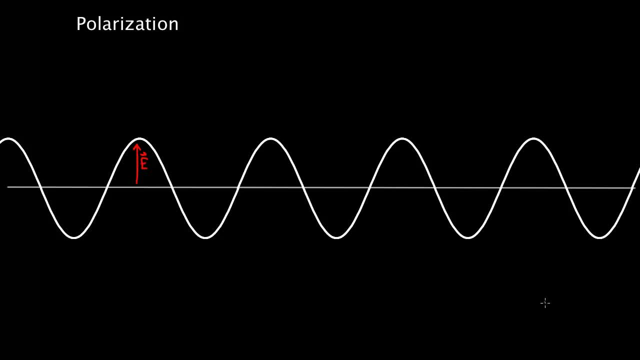 but not in this direction. Let's say, our other light ray had polarization in this direction, so it looks like this Kind of like what our magnetic field would have looked like. but this is a completely different light ray with its own polarization and its own magnetic field. 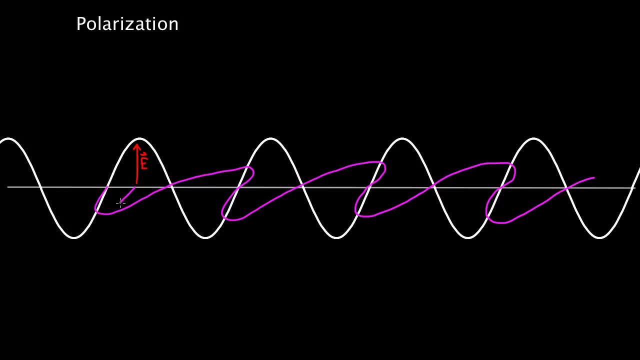 so let's say we sent this in. what would happen? Well, at this point you'd have an electric field that points this way. At this point you'd have an electric field that points that way. What would your eye see if you were over here? 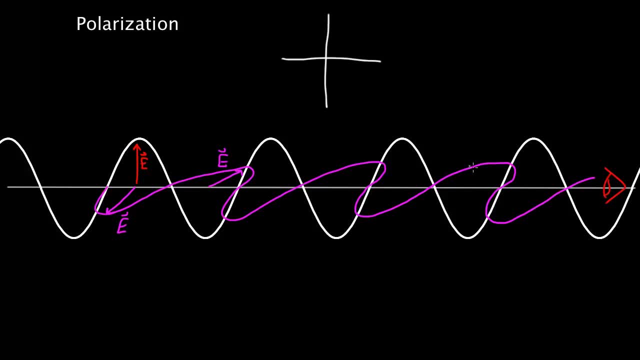 Let's see if I draw our axis here. All right, when this point right here gets to your eye, what am I gonna see? Well, I'm gonna have a light ray. that's one part of the light ray, one component points up. 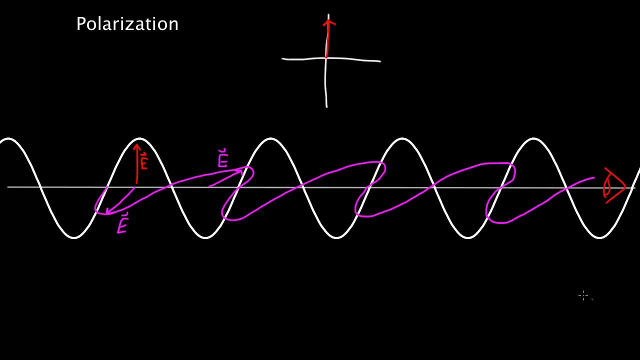 That's this electric field. One component points left. That's this electric field. So the total, my total electric field, would point. this way I could do the Pythagorean theorem if I wanted to figure out the size of it, but I just wanna know. 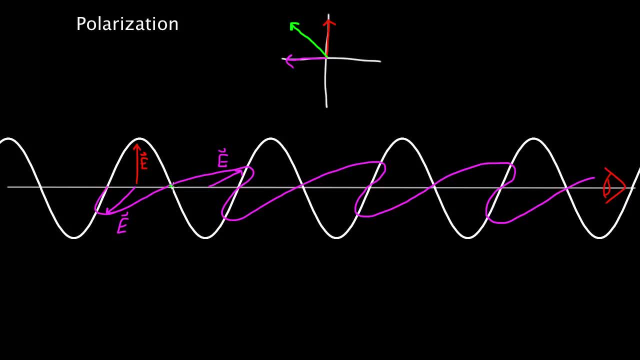 the direction for now. and then it gets to here and look it, they both have zero. This light ray has zero electric field, This one has zero electric field, so then it'd just be a zero. Now what happens over here? 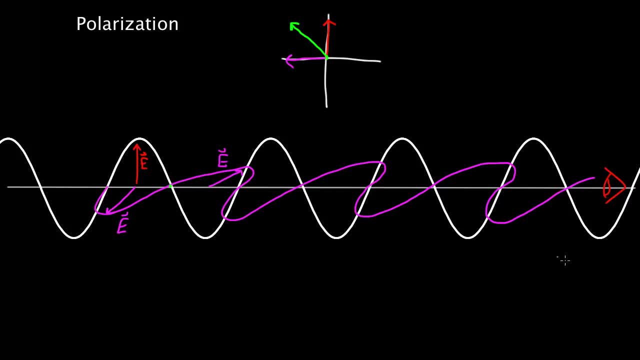 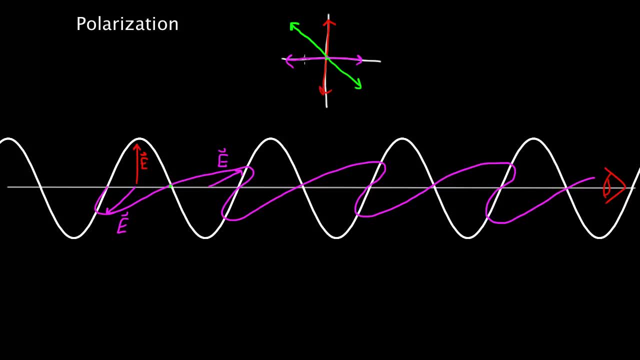 I'd have light that went this way and it would just be doing this over and over. it would just be I'd just have diagonally polarized light. This isn't giving me anything new. You might think this is dumb. 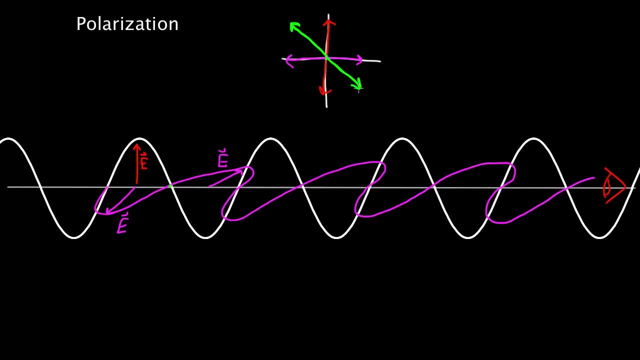 Why do this? Why send in two different waves to just get diagonally polarized light? I could've just sent in one wave that was diagonally polarized and got the same thing. The reason is, if you shift this purple wave, this pink wave, by 90 degrees of phase, 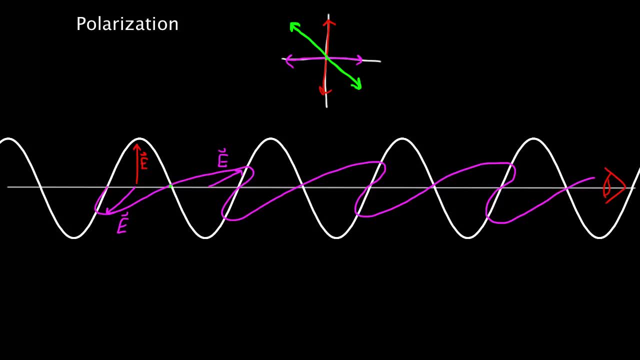 by pi over two in phase, something magical happens. Let me show you what happens here. If we move this to here now, we don't just get diagonally linear polarized light. What we're gonna get is: let me get rid of this. 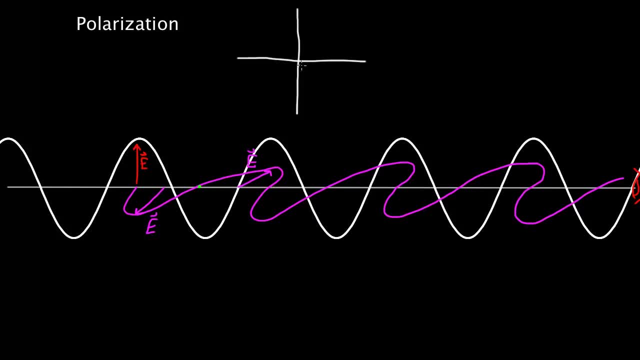 Okay, so we start off with red. the red electric field points up, and then this pink wave's electric field is zero at that point. so this is all I have. My total electric field would just be up. I'm gonna draw it right here. 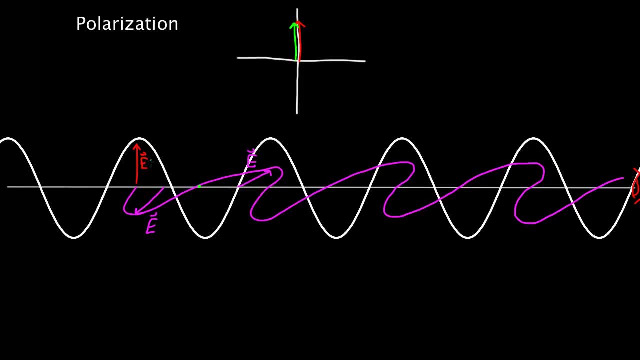 The green will be the total. Now I come over to here, and at this point there's some red electric field that points up, but there's some of this other electric field that points this way, so I'd have a total electric field. 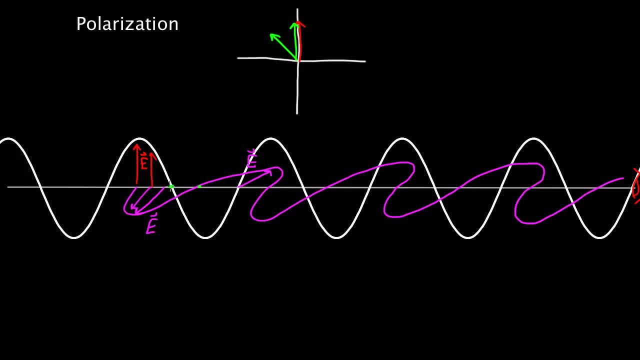 that would point that way. And then I get over to here and I'd have all of the electric field from the pink one, none from the red one. It would point all left. then Look at what's happening, The polarization of this light. if I shift this, 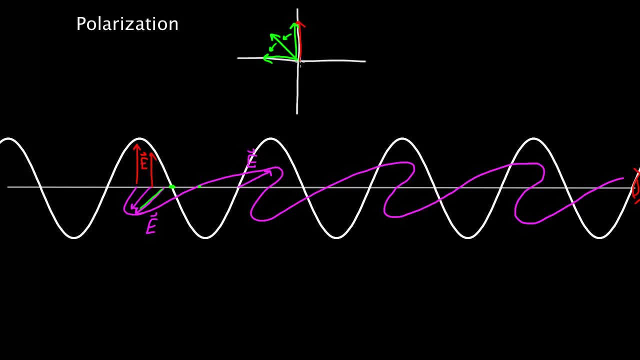 if I'm sitting here looking with my eye, as my eye receives this light, I'm gonna see this light rotate, its polarization, The polarization I'm gonna notice, swings around in this circular pattern and because of this we call this circular polarization. 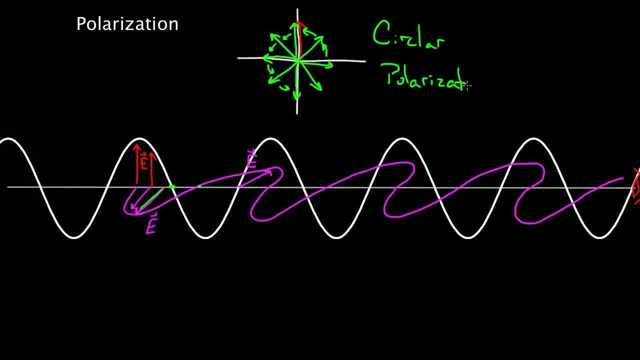 So this is another type of polarization where the actual angle of polarization rotates smoothly as this light ray enters your eye. And you know what er der. all right, actually I said you'd receive this one first. that makes no sense. 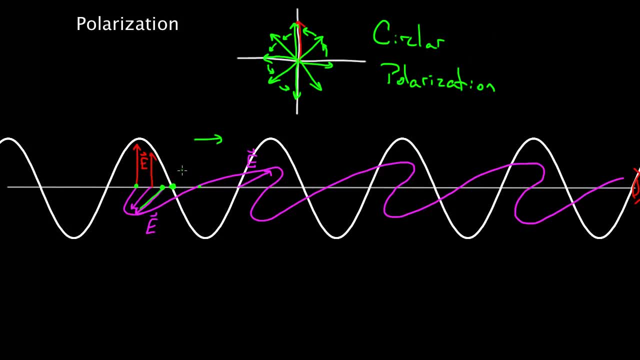 You're gonna receive the ones closest to you first in this light ray going this way. So you'd actually receive this one first, then that one, then this one, then this one. Because of that, you wouldn't see this going in a counterclockwise way. you'd see this going. 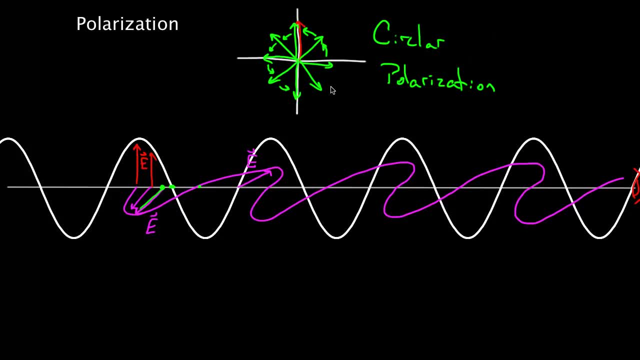 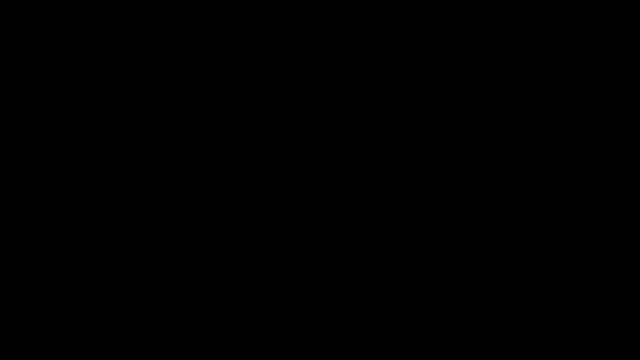 in a clockwise, circularly polarized way. sorry about that. And you might think, okay, why, why even bother with circular polarization? Well, I kinda lied earlier. it turns out in the movie theater example. they don't actually do it. 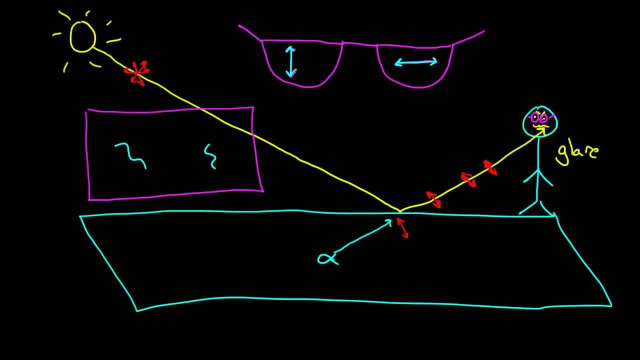 like this. typically, Oftentimes in the movie theaters we don't have just linearly polarized sunglasses. This would be a problem, because when you look at the movie theater screen and if you were to tilt your head just a little bit, think about it. 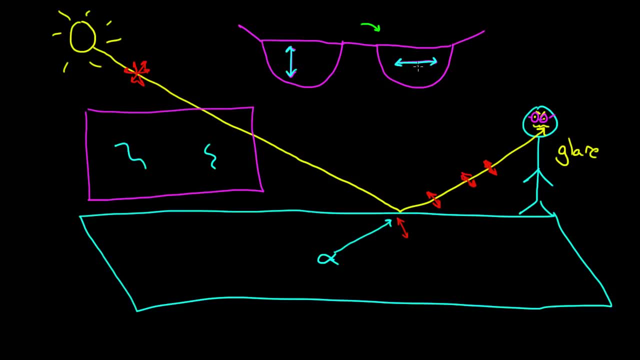 this one's not really gonna get the right image anymore. it's gonna get some of both, and this one's gonna get some of both. it's gonna be blurry. Your head would have to be at perfectly level the whole time, which might be annoying. 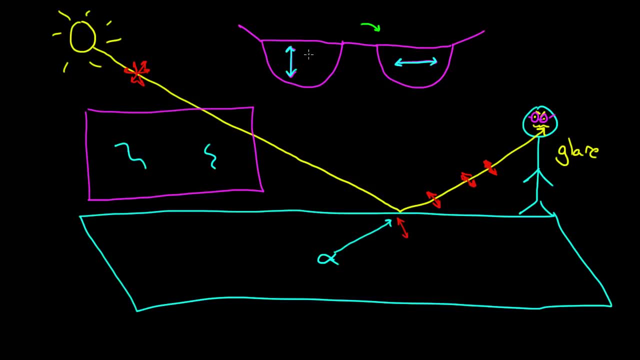 So what we do is instead, we create circular polarized glasses so that this one would only get one polarization, this one would get the other direction. This way, even if you tilt your head a little bit, shoot. clockwise is clockwise, counterclockwise.